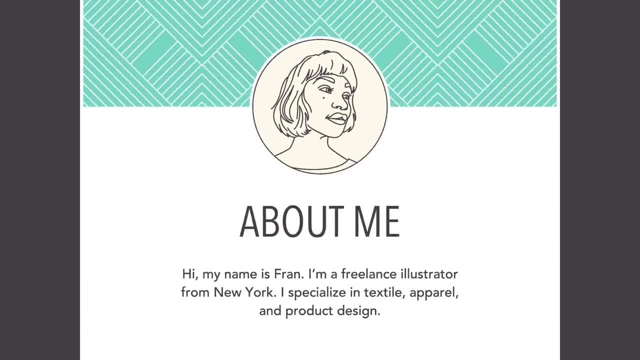 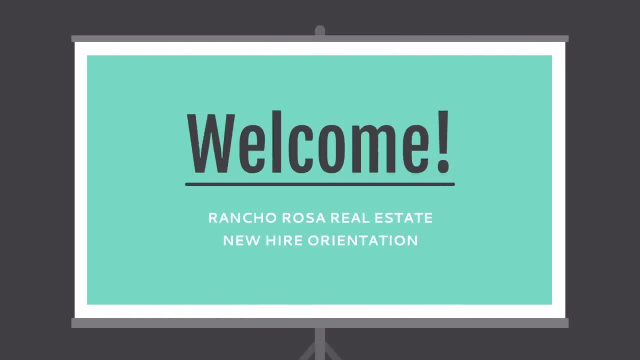 in drawings and illustrations, and graphic elements like textures and patterns. They're also common in text compositions, where they can add emphasis, divide or organize content, or even guide the line. A line can be a shape that connects two different elements. A line- can be a shape that connects two different elements. A line can be a shape that connects two different elements. Politicians perform lines in a different way than they could do with actual characters. This means that they have a different look, shape or change of. 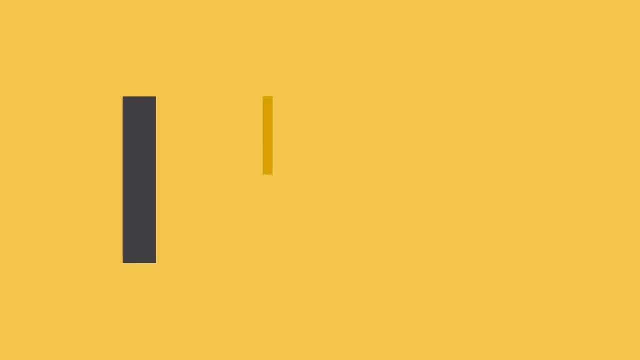 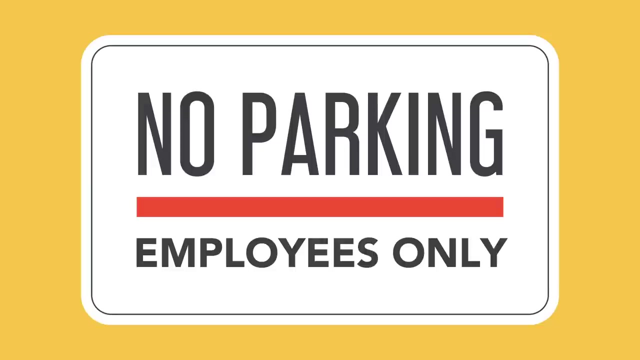 life. as a result, When working with lines, pay attention to things like weight, color, texture and style. These subtle qualities can have a big impact on the way your design is perceived. Look for places where lines are hiding in plain sight, For example, in 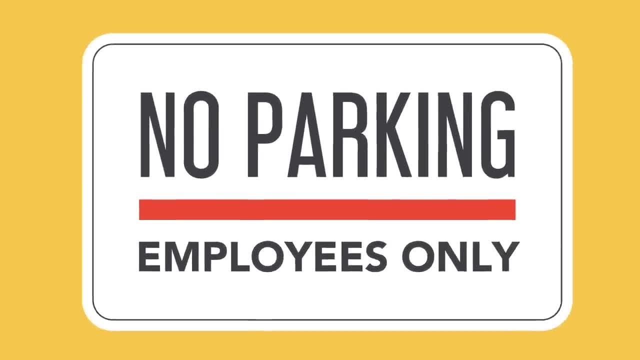 text. Even here, experimenting with different line qualities can give you very different results. These subtle qualities can have a big impact on the way your design is perceived. Here we'll demonstrate some examples of hides- the lines in plain sight- and explain why they. 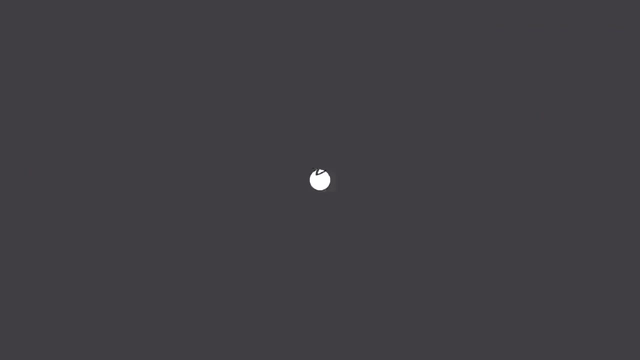 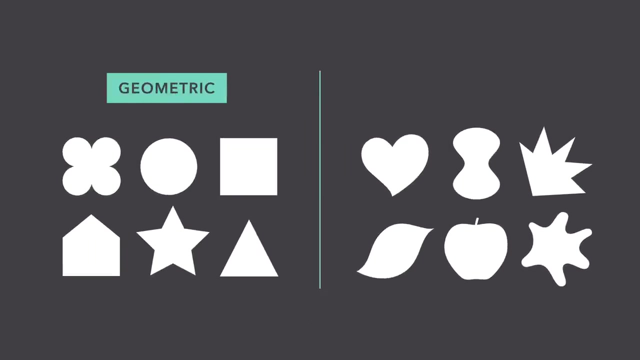 look different really quickly: Legs, neck, vis, bacon or jaw area. Even here, experimenting with different line qualities can give you very different results. A shape is any two-dimensional recognizable boundary. this includes circles, squares, triangles and so on. shapes fall into two distinct categories: geometric or regular, and organic, where 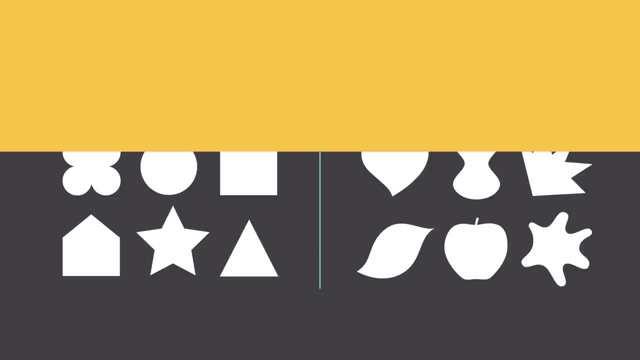 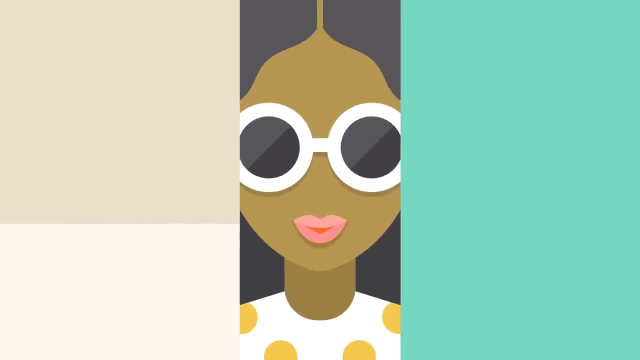 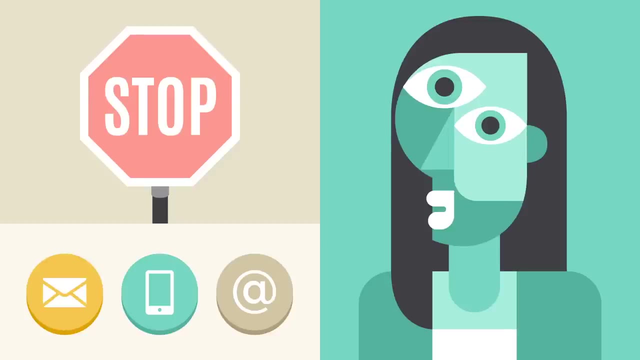 the shapes are more freeform. shapes are a vital part of communicating ideas visually. they give images heft and make them recognizable. we understand street signs, symbols and even abstract art largely because of shapes. shapes have a surprising number of uses in everyday design. they can help you organize or 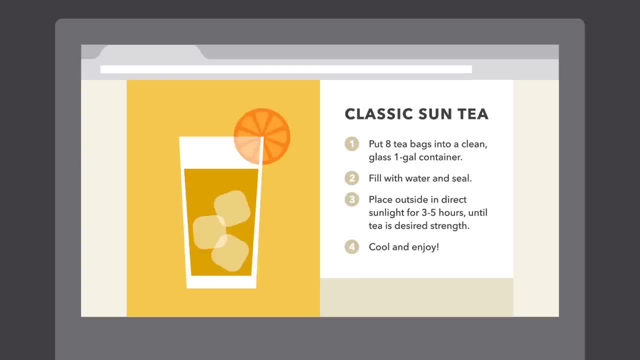 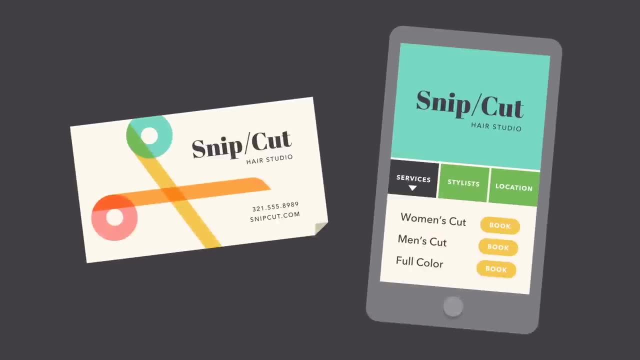 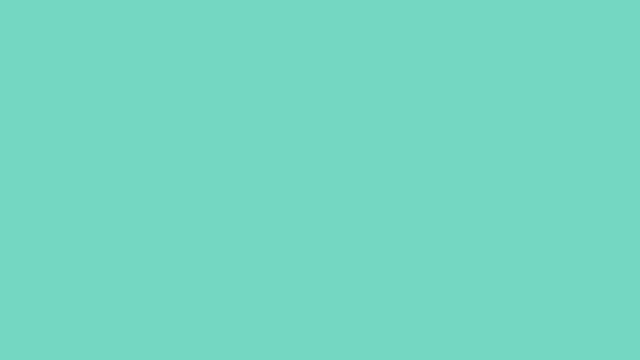 separate content, create simple illustrations or just add interest to your work. shapes are important because they're the foundation of so many things. learn to look for them in other designs and soon you'll start seeing them everywhere. when a shape becomes through 3d, we call it a form. forms can be three-dimensional and exist in the real. 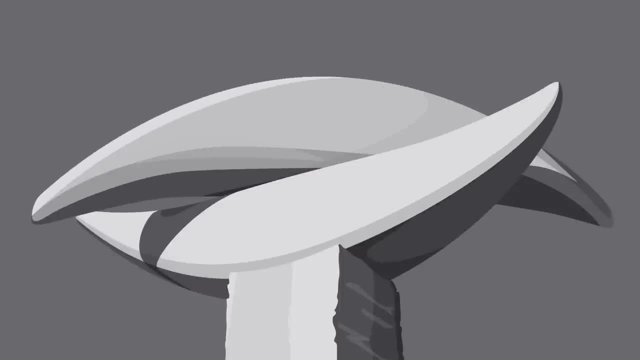 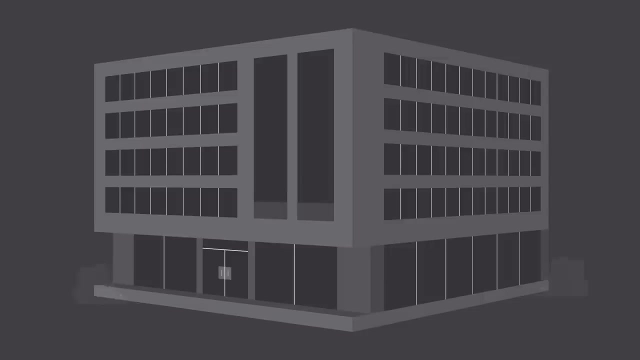 world or they can be implied using techniques like light, shadow and perspective to create the illusion of depth in two-dimensional design form makes realism possible. without it, a bouncing rubber ball is just a circle. a 3d building is just a series of rectangles. even flat designs use subtle 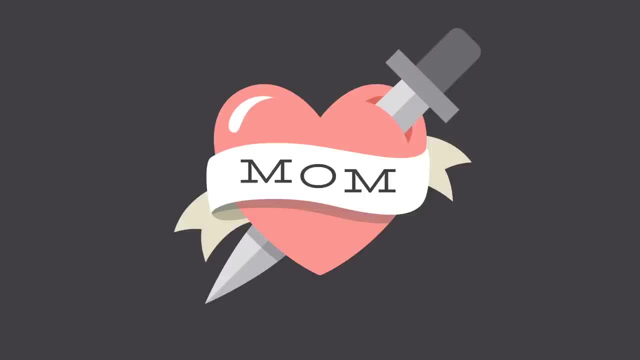 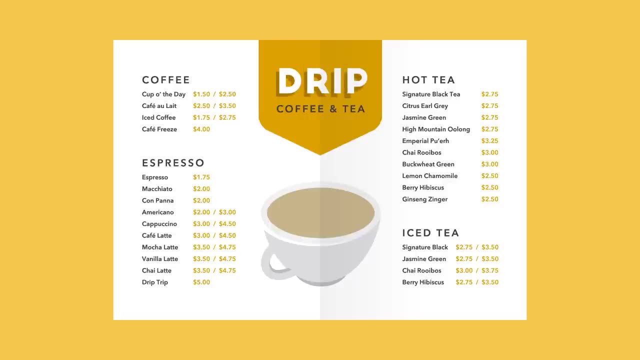 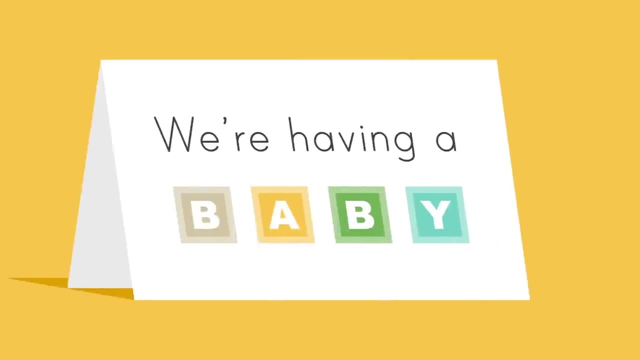 techniques to hint at form and depth and everyday compositions. the purpose of form is the same, but on a smaller scale. for example, a simple shadow can create the illusion of layers or give an object a sense of place. basic forms can bring a touch of realism to your work. a powerful 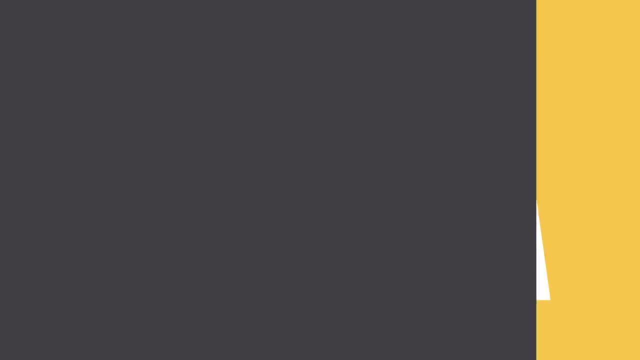 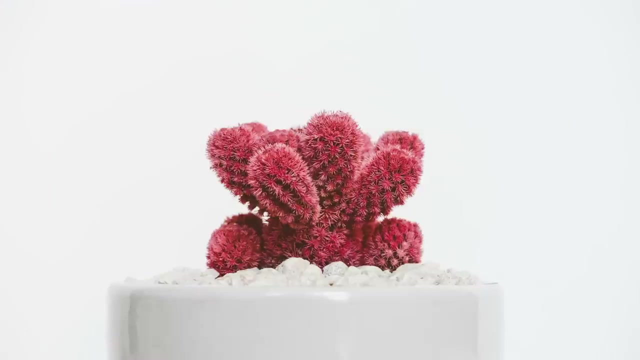 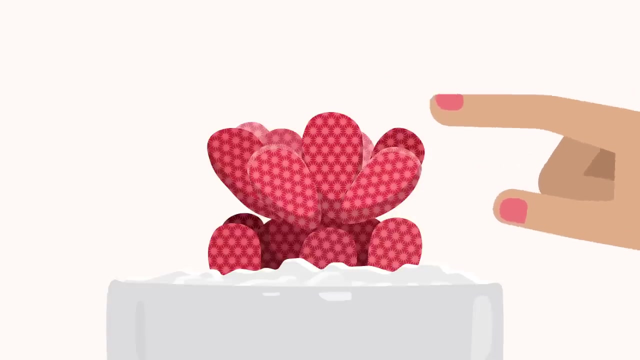 tool when used in moderation. texture is the physical quality of a surface, like form. it can be three-dimensional, something you can see in touch, or it can be 3D, Or it can be implied, suggesting that it would have texture if it existed in real life. 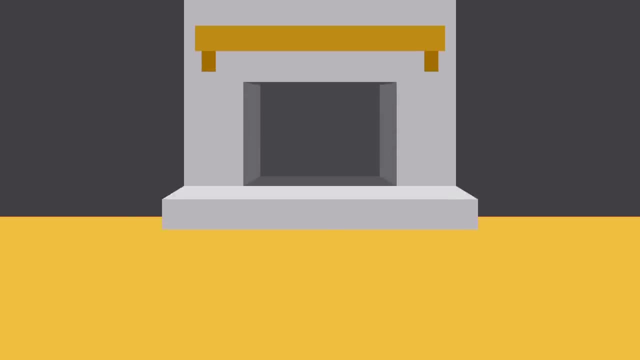 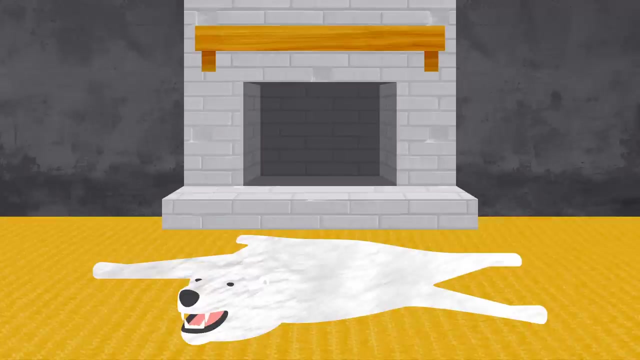 In design. texture adds depth and tactility to otherwise flat images. Objects can appear smooth, rough, hard or soft depending on the elements at play. For beginners, textures make great background images and can add a lot of interest to your work. 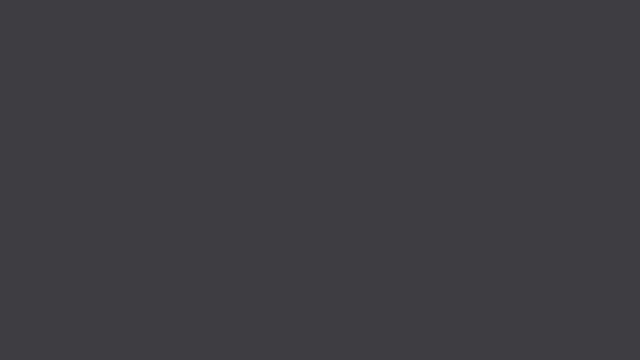 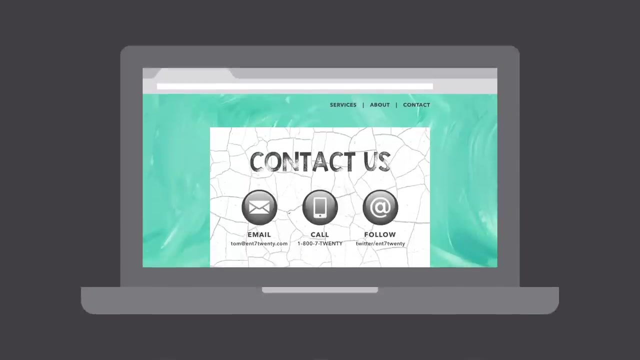 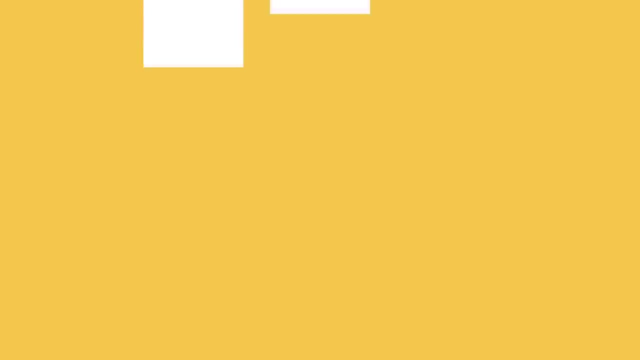 Look closely and you may find texture in unexpected places like distressed fonts and smooth, glossy icons. Just be careful not to go overboard. Too much texture in a single design can quickly become overwhelming. Balance is the equal distribution of visual weight—in other words, how much any one. 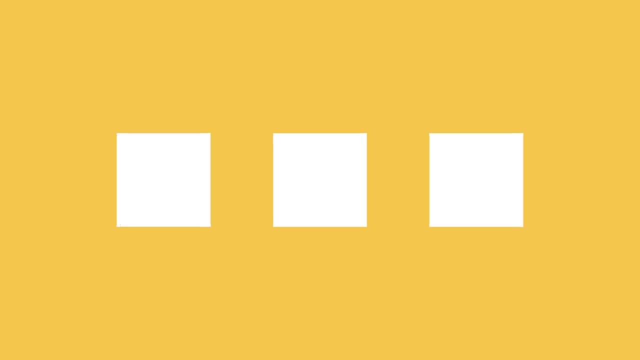 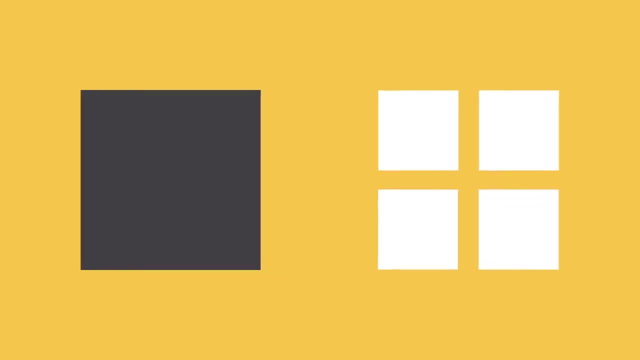 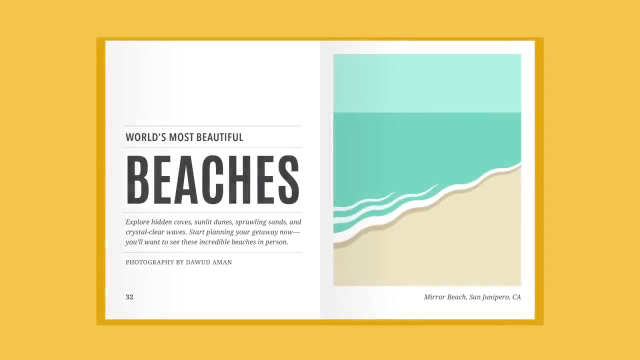 thing attracts the viewer's eye. Balance can be affected by many things, including color, size, number and negative space. Mastering balance can be tricky for beginners, Because it does take some intuition. Luckily, the design world is full of examples that can help you understand its different. 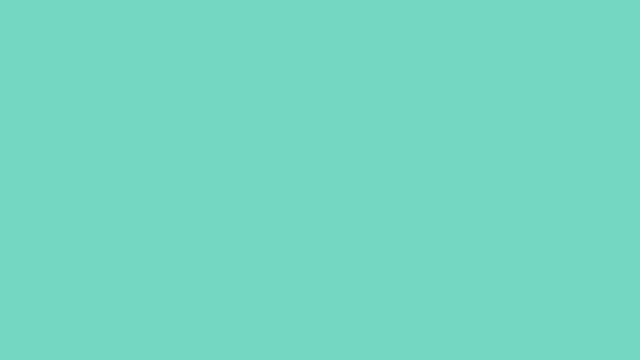 iterations. Symmetrical designs are the same or similar on both sides of an axis. They feel balanced because each side is effectively the same, if not identical. Asymmetrical designs are different, but the weight is still evenly distributed. The composition is balanced because it calls attention to the right things. 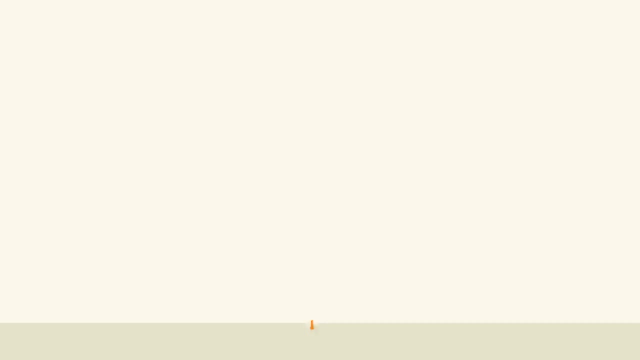 The balance is the same, but the weight is still evenly distributed. The composition is balanced because it calls attention to the right things. The balance is the same, but the weight is still evenly distributed. The composition is just as well. there. The bases and portions of a design.